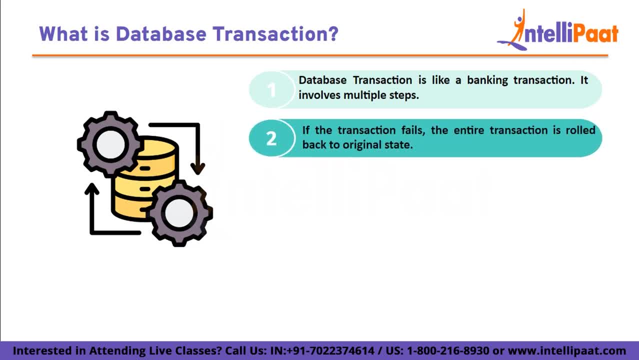 these steps are bundled up together. If any part of the transaction fails, such as insufficient fund for transfer, the entire transaction is rolled back and the database remains at the original state, ensuring data consistency and integrity. Transactions are crucial for ensuring data reliability. 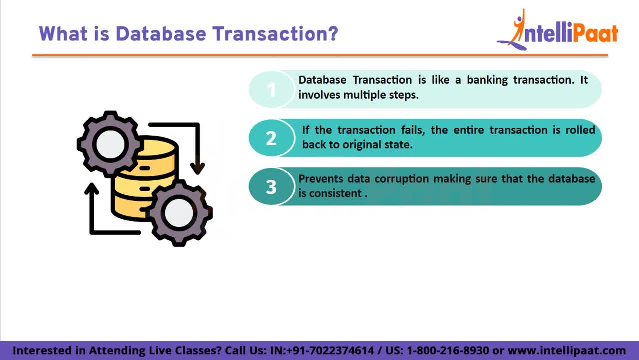 especially in situations where multiple users or processes are accessing and modifying the database concurrently. They help preventing data corruption, incomplete changes or conflict, making sure the database remains in a consistent state even in complex and dynamic environment. In a database transaction, there are typically four different states that a transaction has to go through. 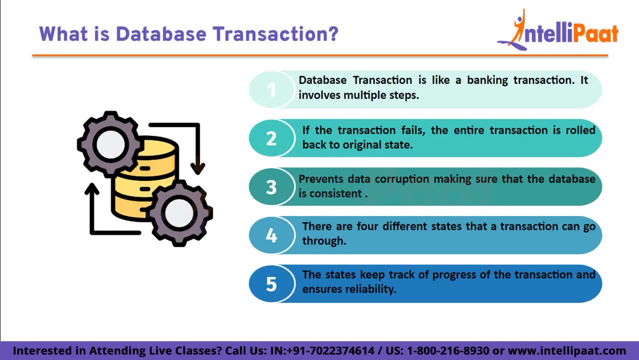 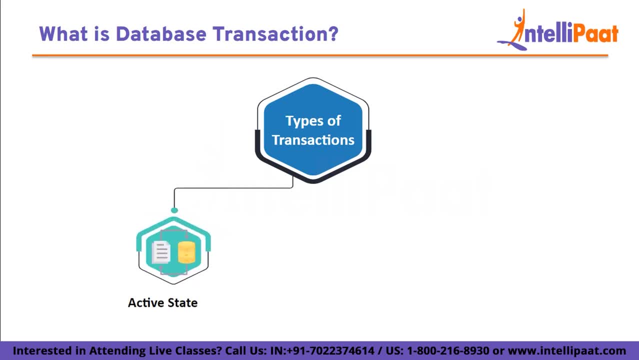 These states are used to keep track of the progress of a transaction and to ensure reliability and consistency of the data. The different states in a transaction are: The first one is active state. This is the initial state of transaction. When a transaction begins, it enters the active state In this state. 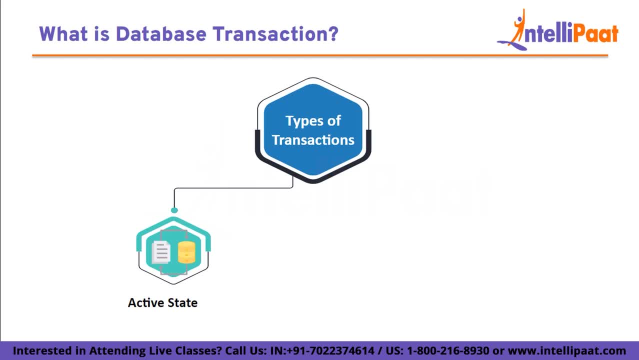 the transaction is actively executing its operations, such as reading data, making changes and performing calculation. During this phase, the transaction is making changes to the database. The next one is partially committed state, After a transaction has executed all its operation and it is ready to make changes permanent. 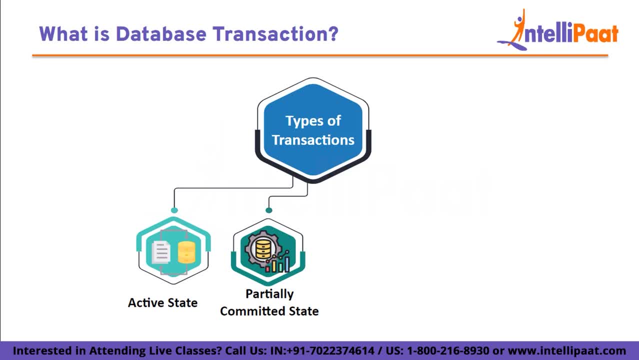 it enters the partially committed state. In this state, the database management system ensures that all the changes made by the transaction are correct and consistent. It checks if the transaction has followed the asset properties and that no rules or constraints have been violated. The next one is committed state. 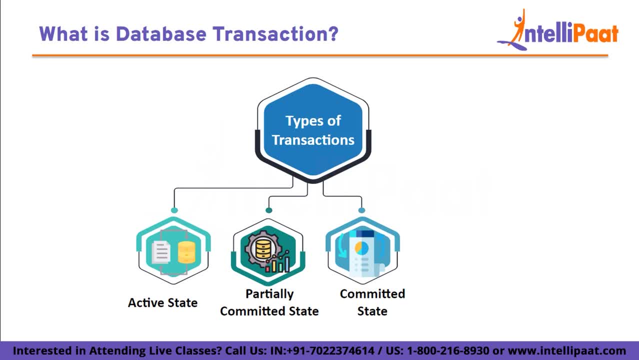 Once the database management system verifies that the transaction changes are correct and consistent, it enters the committed state. In this state the change is made by, the transaction becomes permanent and are saved to the database. Other transaction can now see and use these changes. The transaction is considered successfully completed. 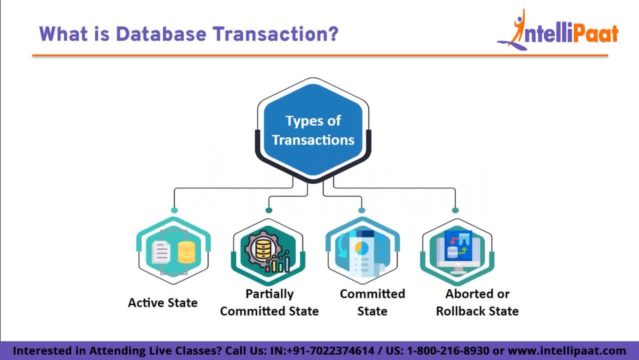 The last one is aborted or a rollback state. If, at any point during its execution, If a transaction encounters an error or violation of a database rule, it may enter the aborted or rollback state. In this state, all the changes made by the transaction are undone or rolled back. 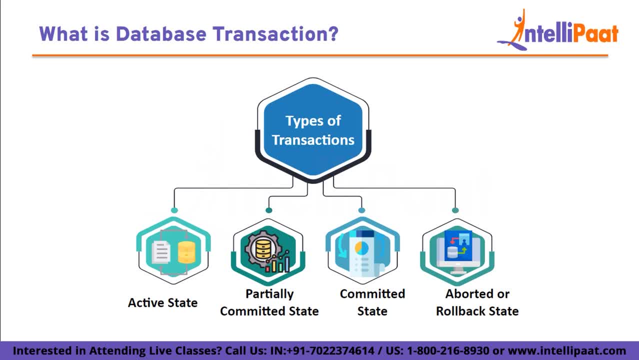 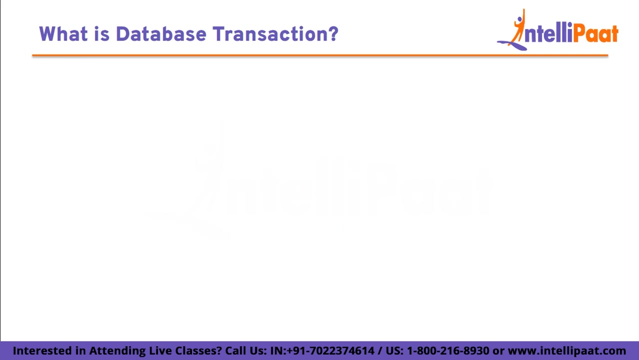 The database is restored to the previous state, as if a transaction never occurred. This ensures that the database remains in a consistent state even if a transaction fails. These transaction states help in ensuring data integrity and consistency within a database system. They also allow to recover in the cases of error or failure, preventing data corruption and maintaining the reliability of the database. 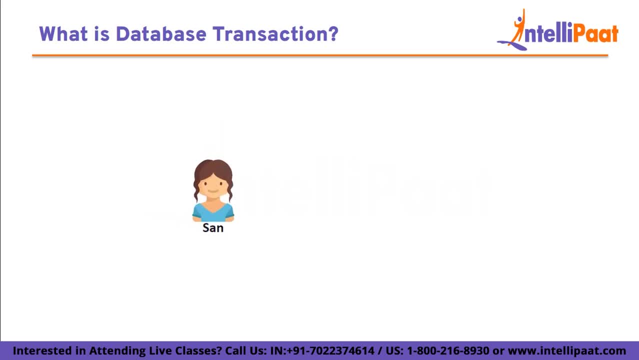 Consider: San wants to transfer Rs 1000 from her account to Rohit's account. San tells the bank that she wants to transfer Rs 1000 to Rohit. This marks the beginning of a transaction. The bank checks San's available balance, which is Rs 5000. 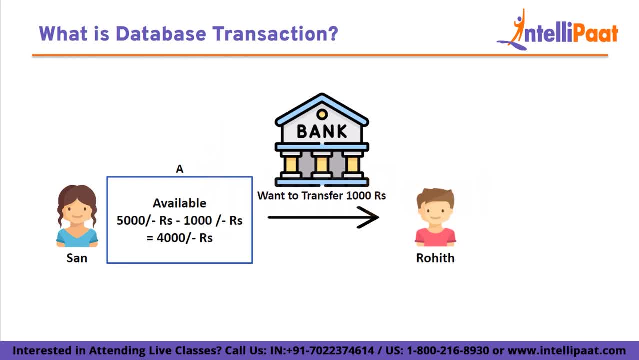 The bank subtracts Rs 1000 from San's account, leaving her account with Rs 1000.. The bank checks Rohit's balance, which is currently Rs 2000.. The bank adds Rs 1000 to Rohit's bank account, making his balance Rs 3000. 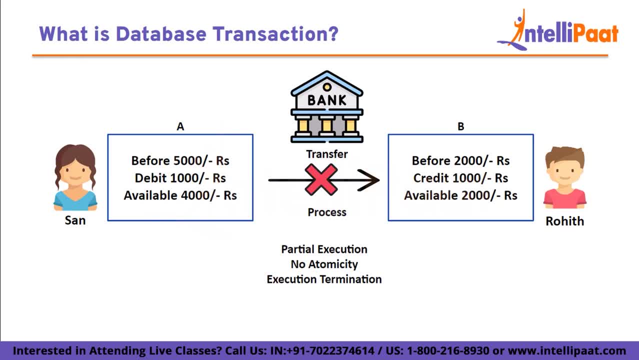 Now, let's say there is a sudden power outrage and the transaction is interrupted. In this case it's like erasing all the changes made during the transaction: San's balance goes back to Rs 5000 and Rohit's balance remains at Rs 2000.. 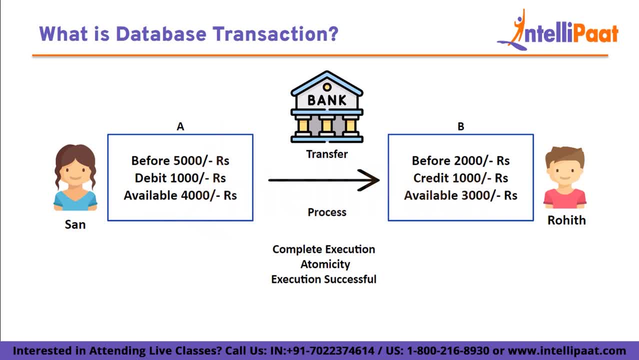 If a transaction is completely successful, San's balance stays at Rs 4000 and Rohit's balance is Rs 3000, the transaction is now permanent. So a database transaction ensures when Rohit and San engages in the financial exchange, either everything happens as intended or no changes happen at all. 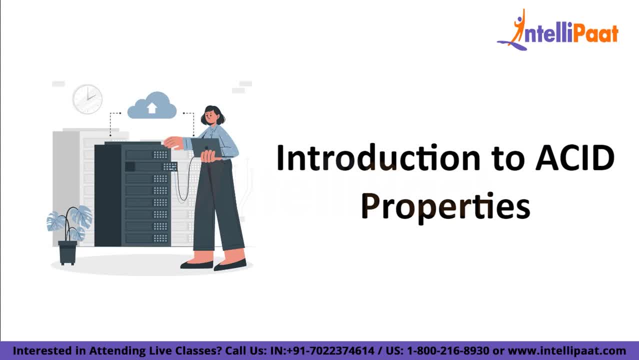 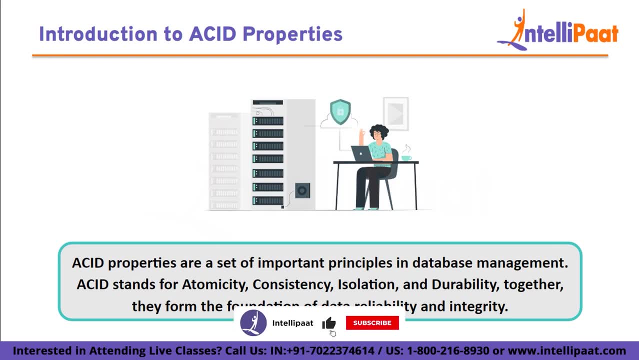 So the next topic is introduction to asset properties. Asset properties are a set of important principles in database management system. Asset stands for Atomicity, Consistency, Isolation and Durability. Together they form a foundation of data reliability and integrity. Asset properties primarily ensure that the data stored in a database is trustworthy, accurate. 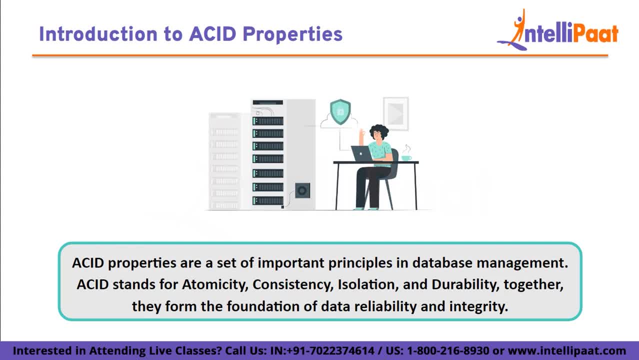 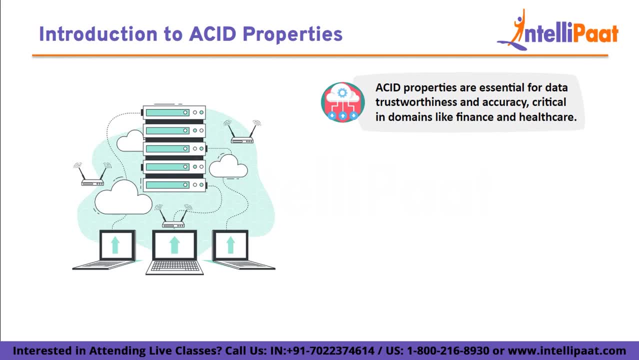 regardless of how complex and demanding the operation performed on them may be. Asset properties are vital because they provide a safe net to data, ensuring that it remains intact, consistent and reliable. This level of data integrity is critical in various domains: for financial systems, where accurate transactions are essential, to healthcare, where patient records must be safe and precise. 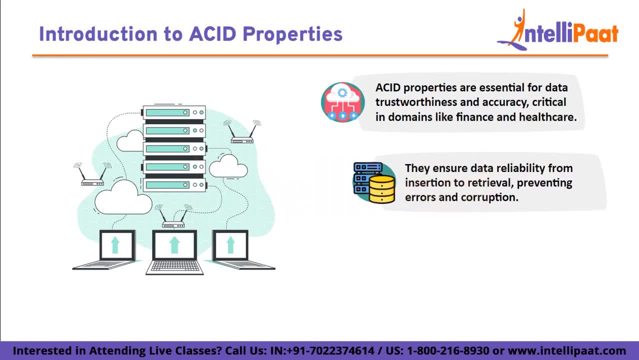 Without asset properties, the trustworthiness of data would be compromised, leading to errors, inaccuracies and potential disastrous consequences. Therefore, asset properties are the core of ensuring the quality and dependability of data in database management system. Now let's consider a scenario to understand asset property better. 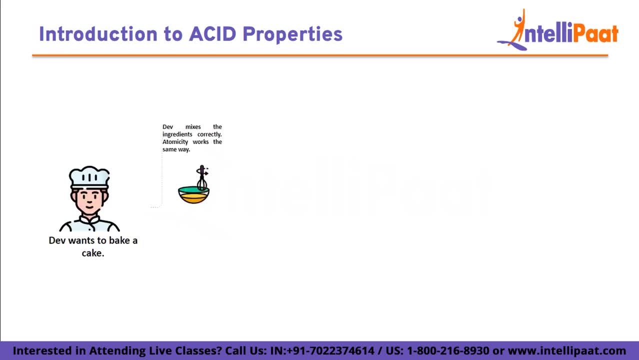 Imagine Dave wants to bake a cake. Dave mixes the ingredients for the cake. Either he mixes them completely or he does not mix them at all. Atomicity works the same way, ensuring to complete each step fully to get delicious cake. If a recipe says use one cup of sugar, 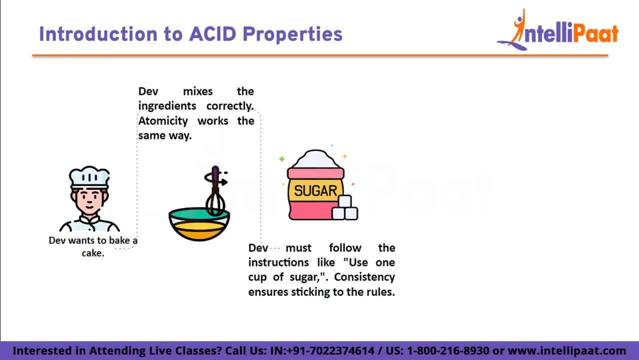 Dave does not suddenly decide to use three cups. Consistency ensures sticking to the rule, So his cake always tastes the same and turns out as expected. In a busy kitchen he might have family members helping with different tasks. Isolation is like making sure each person is responsible for the part of cake making process. 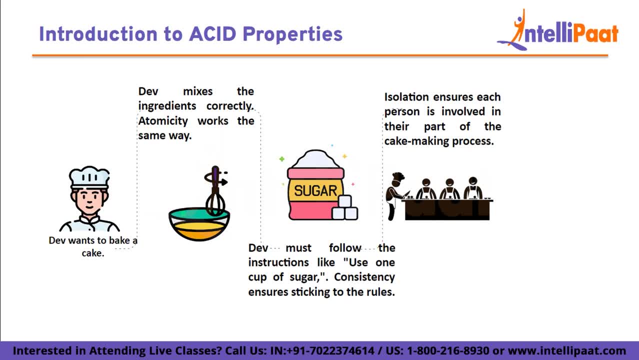 His sister cannot accidentally pour salt into the batter when he is not looking into, because a task is isolated from his Durability is about making sure the cake does not fall apart after it has been baked, Once it is out of the oven and cooled down. 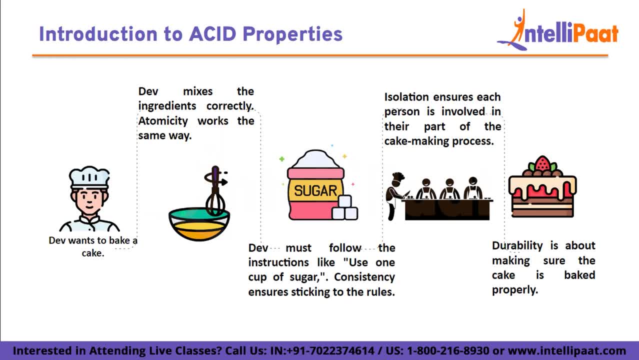 it should remain delicious and intact, even if it is accidentally bumped into or the power goes off. Durability ensures that the cake stays yummy and does not crumble easily. So asset properties just follow the right steps, as in baking, Making sure that the actions involved in data are completely consistent, without interference. 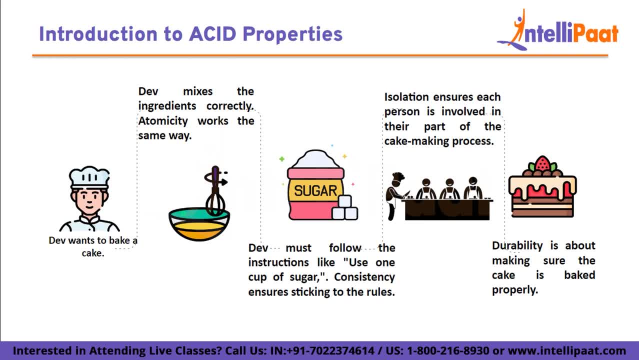 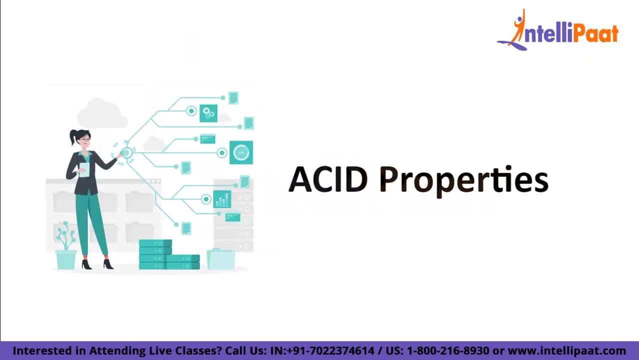 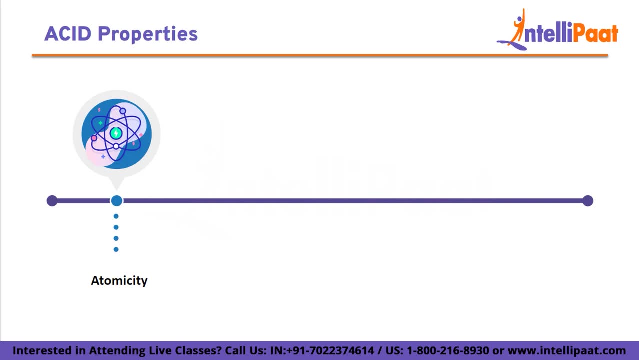 Asset properties are similar to following a recipe in baking a perfect cake. So the next topic is asset properties. The first property is Atomicity. In a database transaction, Atomicity is one of the key properties that ensure that all the actions within a transaction are treated as a single unit. 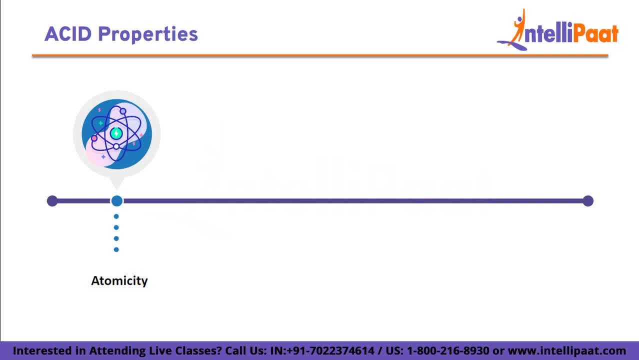 Atomicity guarantees that either all the operations within a transaction are successfully completed or none of them are. There is no in-between state. If any part of the transaction fails, the entire transaction is rolled back or cancelled. This means that any changes made to the database during a transaction are undone. 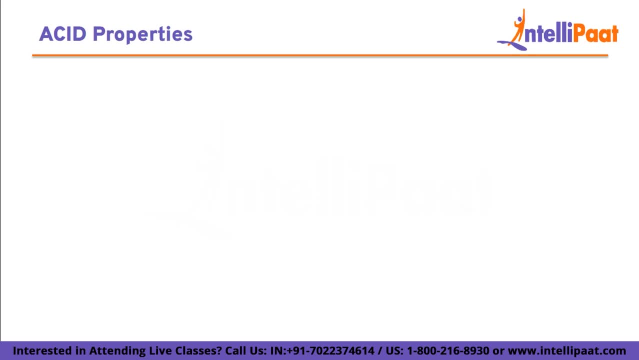 and the database returns to its original state. Consider: Bob orders a pizza online. He chooses the pizza he wants, adds some toppings and click on order. Atomicity is like a promise that all the choices- the type of pizza, the toppings and the order itself- will be completely perfect or none of them will happen. 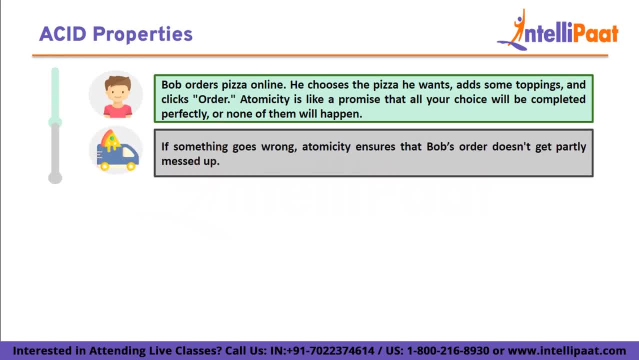 If something goes wrong, like the internet connection fails, Atomicity ensures that Bob's order does not get partially messed up. It undoes everything, so that he does not end up with a half payment or half pizza. Either Bob gets the complete order or it's like nothing happened. 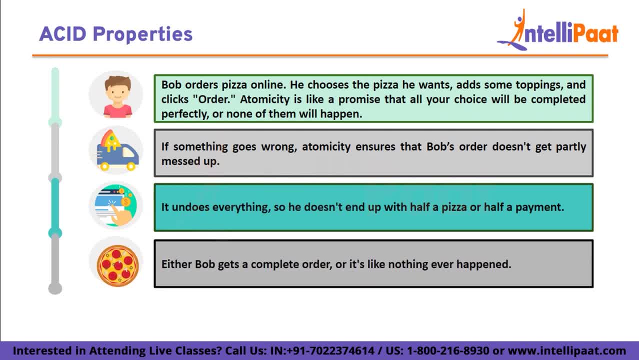 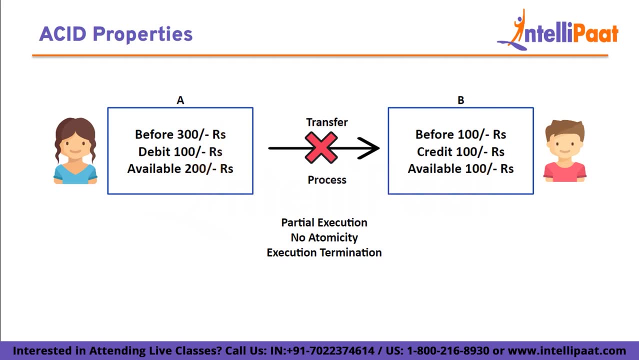 So in a database, Atomicity is an action that will either happen entirely or nothing will happen at all: making sure that the data stays accurate and safe, just like Bob's pizza order. Consider if San has an account having 300 rupees from which he wishes to send 100 rupees to Rohit's account, which is B. 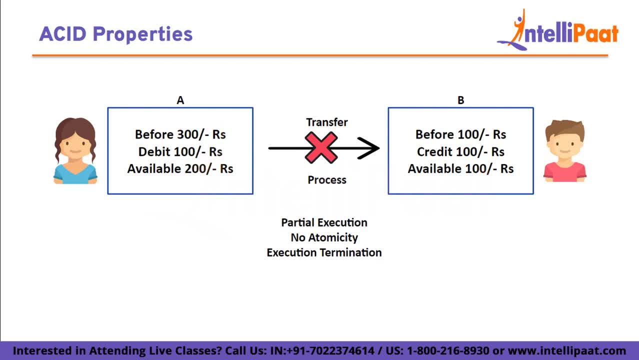 In account B, a sum of 100 rupees is already present. When 100 rupees will be transferred to account B, the sum becomes 200.. Now there will be two operations that take place. One is that the amount- Rs 100- that San wants to send will be debited from our account. 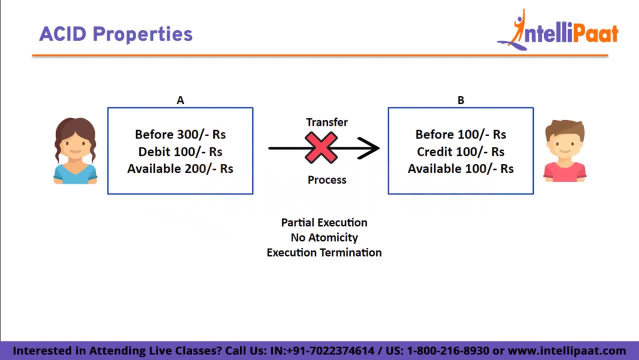 and the same amount will be credited to the account B, That is, Rohit's account. Now what happens is the first operation of debiting is executed successfully, But the crediting operation somehow fails. Thus, San's account, the value becomes 200 and Rohit's account, it remains 100. 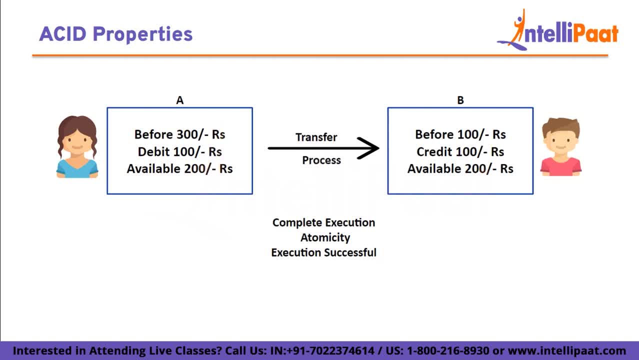 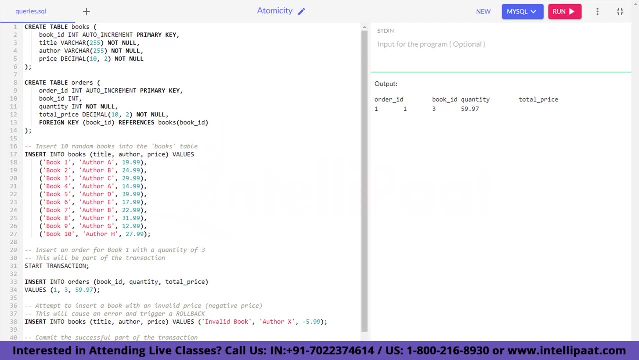 So it is not in an Atomic transaction. If both the debit and credit operation are done successfully, then the transaction is Atomic. We consider two tables: Books and Order. The book table stores the information about the books and the other order table stores the information about the customer's order. 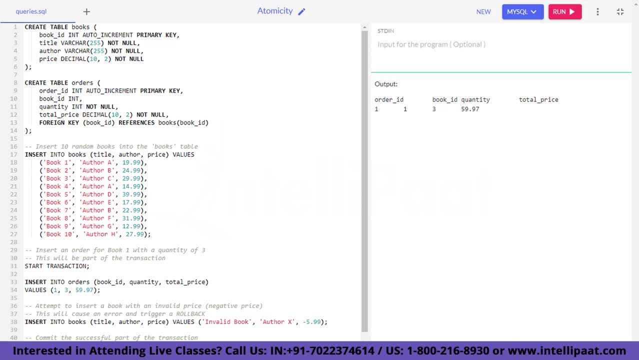 The order table have a foreign key constraint referring to the Book ID column in the book table, establishing a relationship between the two tables, And then we insert different books with the title, author and the name, Then we add the price to the books table. 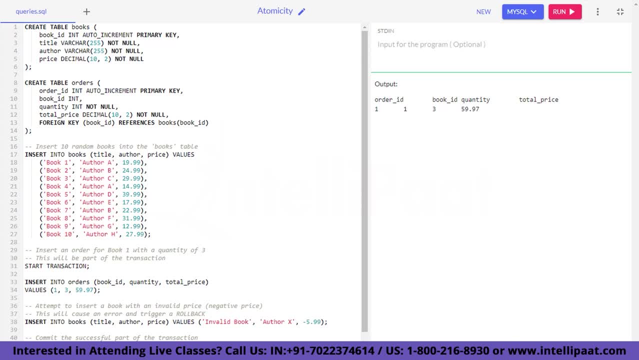 Once we are done with that, we initiate a database transaction using a start transaction statement. Within the transaction we insert an order for Book 1 with the quality of Book 3. This step is successful and is a part of the ongoing transaction. 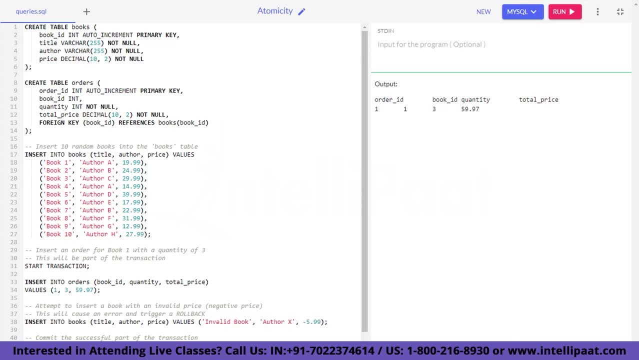 Later we attempt to insert the new book with an invalid price. This action triggers an error due to the database constraint, causing the transaction to be in an inconsistent state As a result of error. we explicitly roll back the transaction using the rollback statement. This action ensures that all the changes made within a transaction 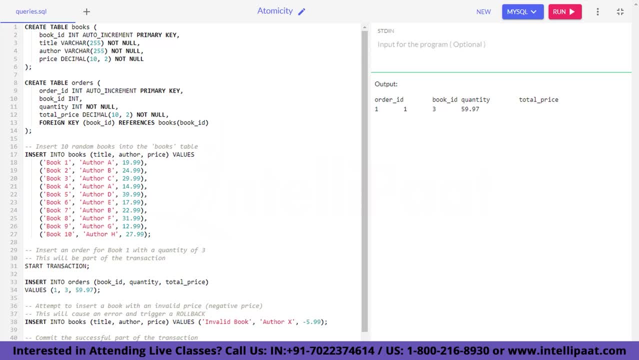 including the insertion of the order Book 1, are undone, The database returns to the previous state. Since the transaction was rolled back to the previous state, we do not execute the comment statement. The transaction remains in the aborted state. We then verify the book order. 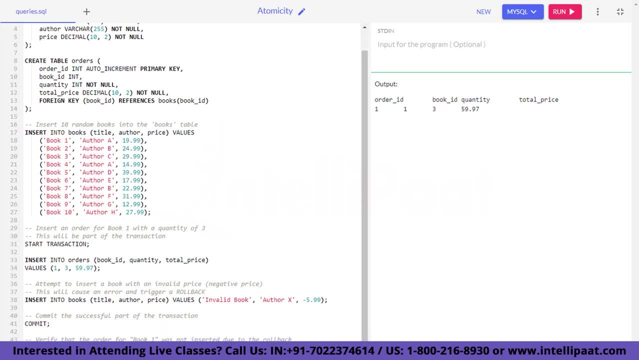 The order for Book 1 was not inserted due to the rollback. Finally, we perform the SELECT statement to check the content of the order table. Because the transaction was rolled back, the order for Book 1 is not present in the table demonstrating the atomicity property of a database transaction. 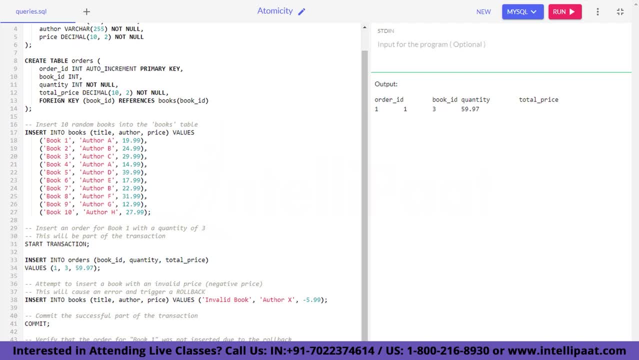 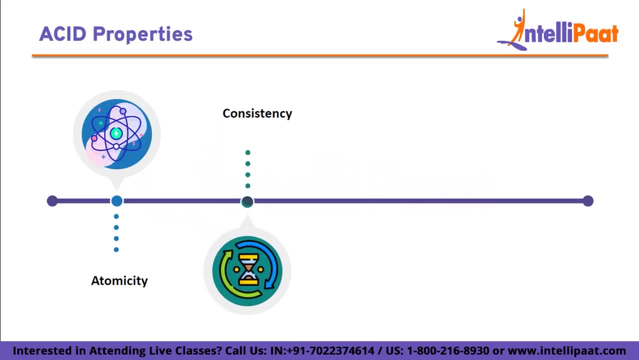 All changes made either to the transaction were applied together or not applied at all, ensuring data consistency and integrity. So the next property is Consistency. In a database transaction, consistency is one of the key property that ensures your data remains in a valid and a stable state. 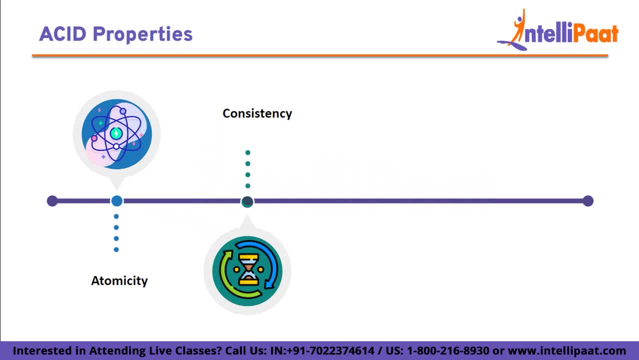 even as changes are made during the transaction. Consistency ensures that the data follows all the rules and consistency defined in a database. These rules can include things like ensuring unique value, enforcing data types or verifying the certain conditions are met During a transaction. any changes made to the database. 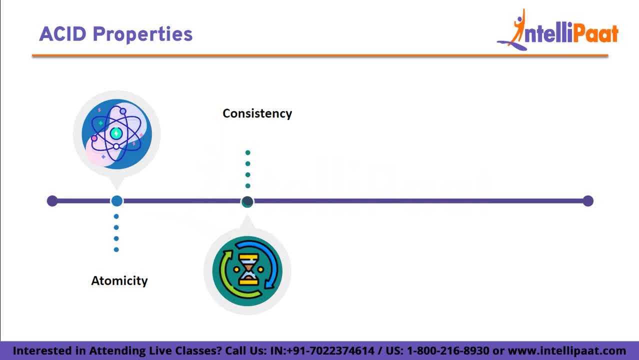 must follow these predefined rules At any point. a change is violated to the rule, the transaction is rolled back and the database remains unchanged. This ensures that the data stays consistent with the established standard. Consistency in database is like making pizza. Consider Bob ordering his favorite pizza again. 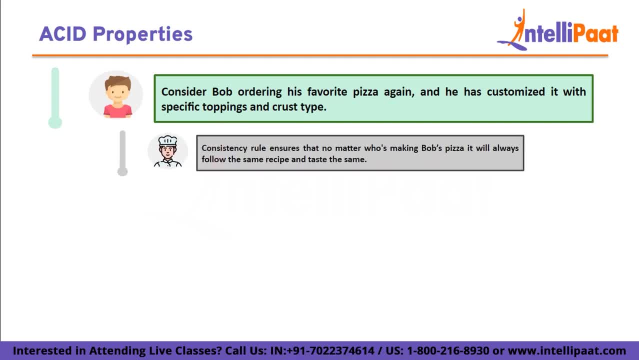 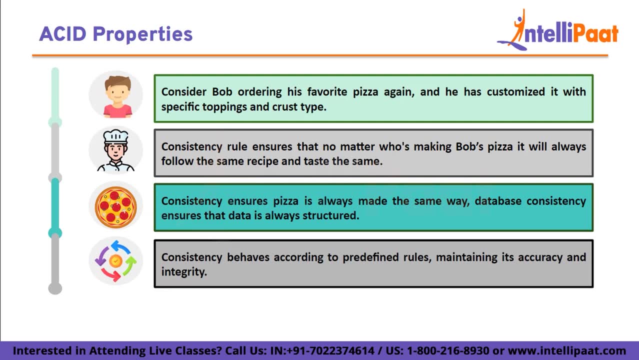 He has customized it with a specific topping and crust type. Consistency rule ensures that no matter who makes Bob's pizza, whether it is made in New York or California, it will always follow the same recipe and tastes the same. So just like consistency rule in pizza making. 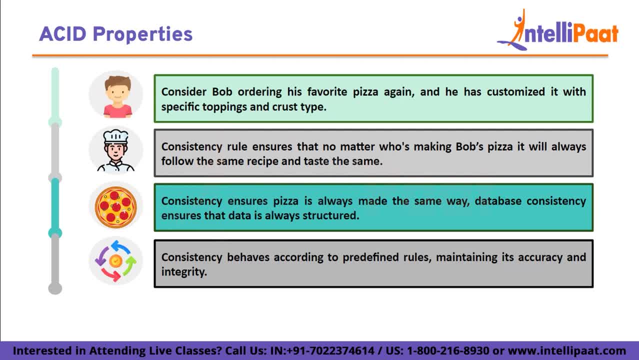 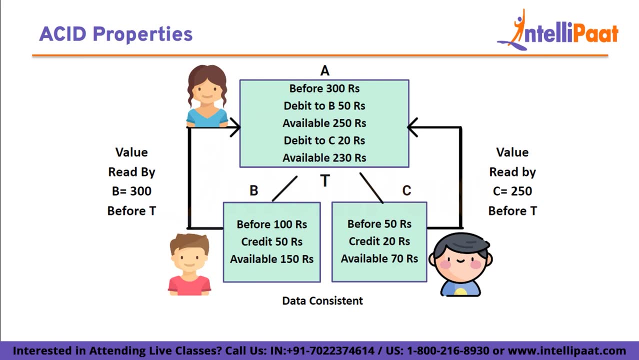 ensuring pizza is always made the same way. database consistency ensures that the data is always structured and behaves according to the predefined rules, maintaining its accuracy and integrity. Let's say there are three accounts- A, B and C, where A is making a transaction T one by one to both B and C. 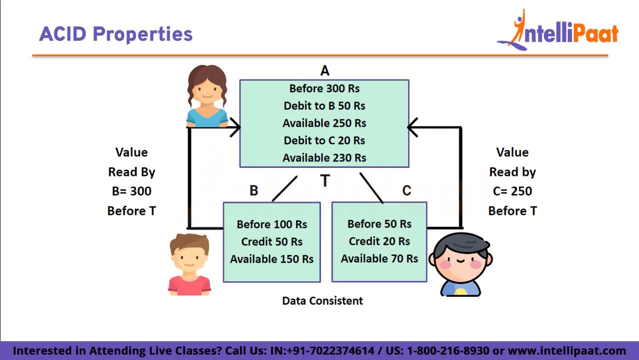 There are two different operations that take place: debiting and crediting. Account A firstly debits 50 rupees from account B and then the amount in A is read 300 by B before the transaction. After successful transaction T, the available amount in B becomes 150 rupees. 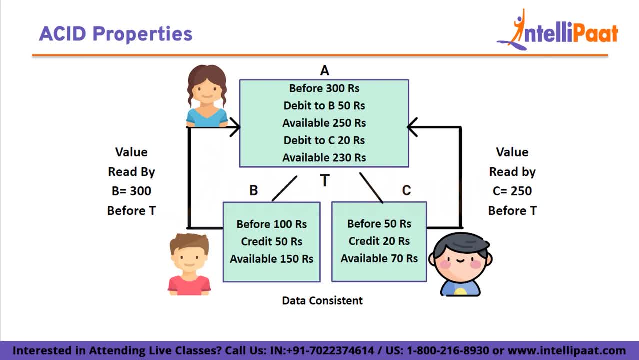 Now A debits 20 rupees to account C and that time the value read by C is 250 rupees. The debit and credit operation from account A to C has been done successfully. We can see that the transaction is done successfully and the value is also read correctly. 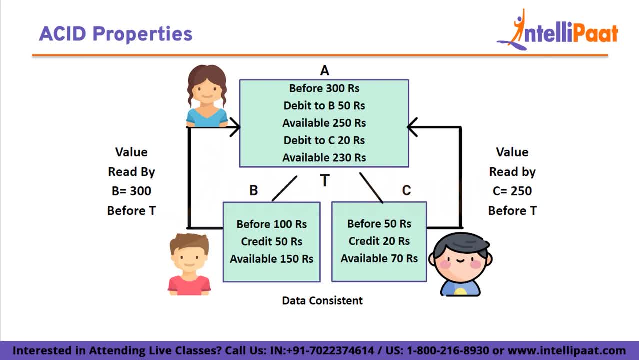 Thus the data is consistent. In this case, the value read by B and C is 300, which means that the data is inconsistent because when the debit operation executes it will not be consistent. Here we have a transaction involving two related tables: order and the order item. 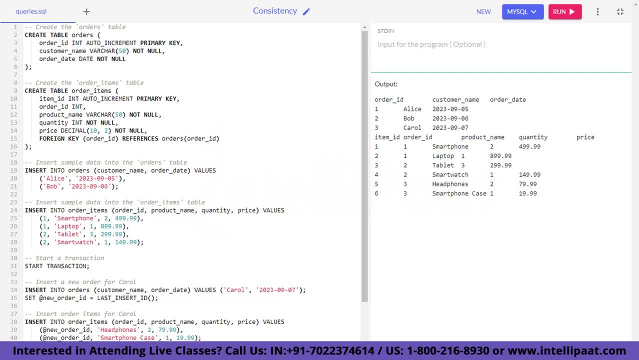 We insert item Carol's order into order item table. If all the SQL statements within a transaction are successful and execute without error, we commit the transaction using a commit statement. This finalizes the transaction and makes all the changes made permanent in a database. 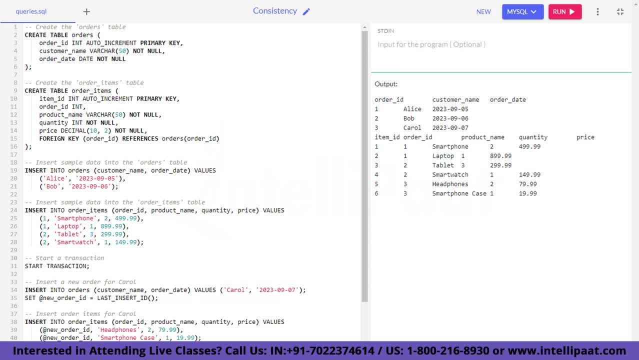 It's a critical point here that a transaction ensures data consistency. If any point of transaction were to fail, the rollback statement could be used instead of commit to cancel all the changes made during the transaction. This prevents the database from being left in an inconsistent state. 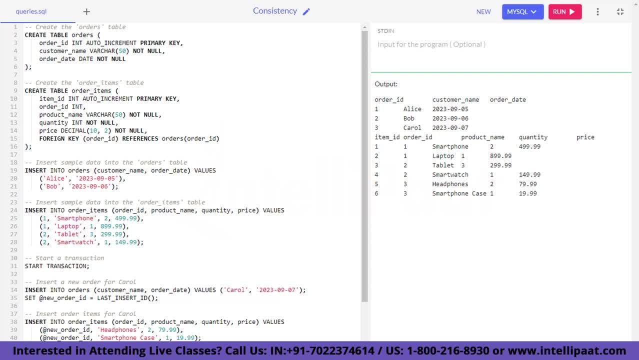 By using a transaction, we guarantee that either all the operations within a transaction successfully complete together or fails together, maintaining the integrity and consistency of the data. This is crucial in scenarios like online orders, where you want to ensure both the order and its associated items. 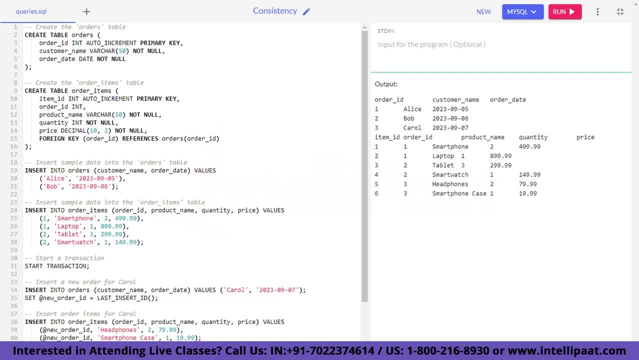 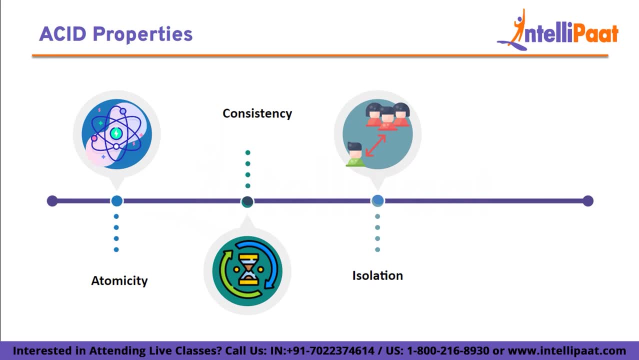 are correctly recorded in the database or not recorded. The next property is Isolation. Isolation refers to a property that ensures each transaction is isolated or separated from others. It means that even when multiple transactions are happening simultaneously in a database, they should not interfere with each other. 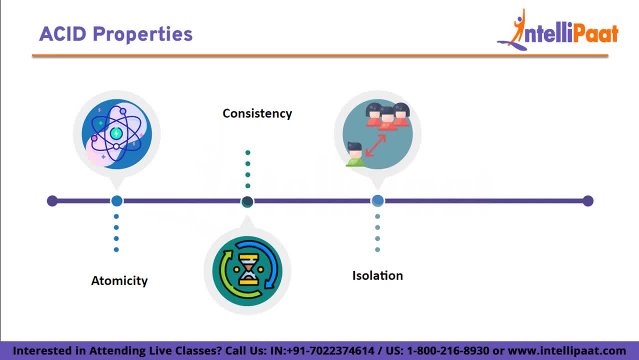 or produce inconsistent results. Isolation ensures that if two or more transactions are running concurrently, they should behave as if they are running concurrently. This means that if two or more transactions are running concurrently, they should behave as if they are happening one after the other. 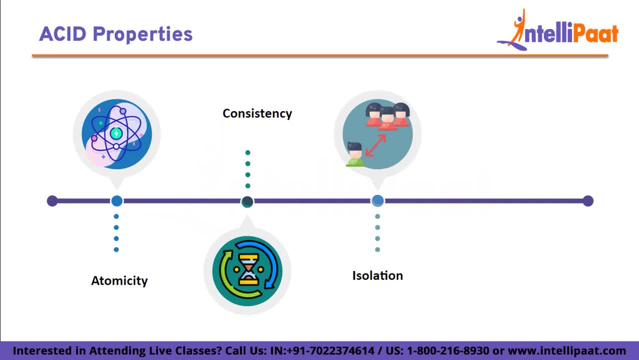 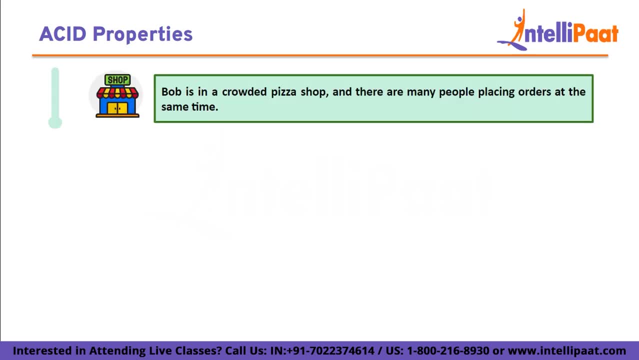 not simultaneously. This prevents data conflicts, inconsistency and error that could occur if a transaction were allowed to interfere with each other. Isolation in a database is like having a separate chef who is preparing your order separately, So no one else can interfere with Bob's pizza while it is being made. 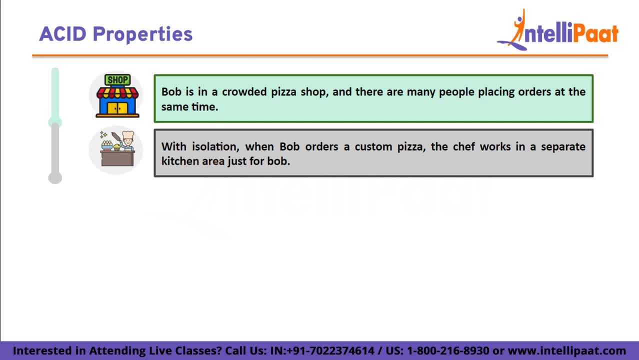 Imagine Bob is in a crowded pizza shop and there are many people placing order at the same time, With Isolation. when Bob orders a customized pizza, the chef works on a separate kitchen area just for Bob. This way, no matter how busy the shop is, 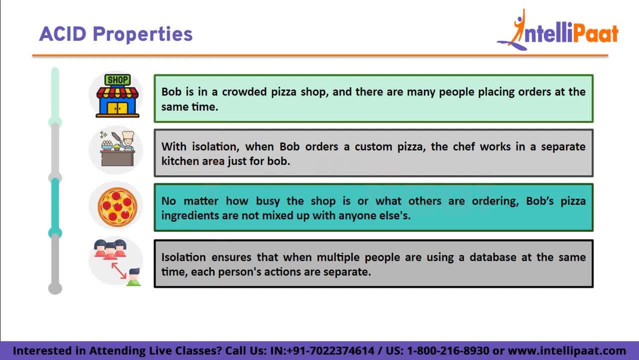 or what others are ordering Bob's pizza ingredients are not mixed up with anyone else In a database. Isolation ensures that when multiple people are using the database at the same time, each person's actions are separate. It's like making sure Bob's pizza order does not get mixed up with someone else's. 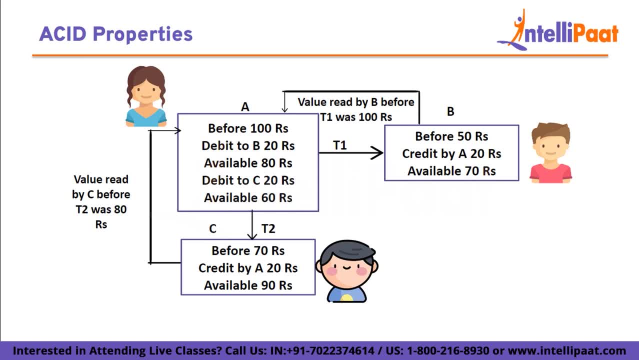 Consider two operations. Consider two operations are concurrently running on two different accounts, Then the value of both the accounts should not get affected. The value should remain persistent. As you can see, account A is making T1 and T2 transaction to account B and C. 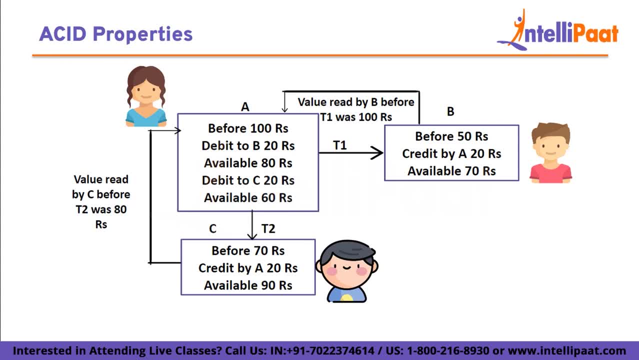 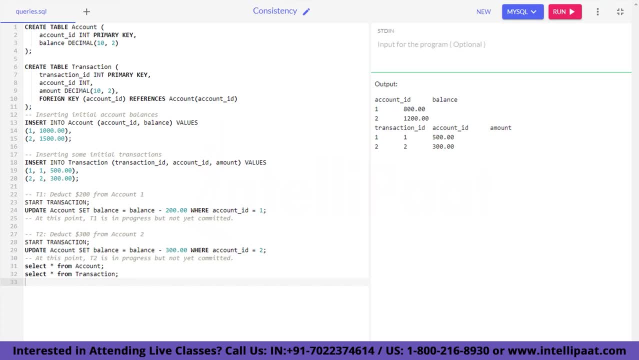 but both are executing independently, without affecting each other. This is known as Isolation. We consider two transactions, T1 and T2, being executed concurrently. We define two database table- Account and Transaction- which will be used to stimulate bank account transaction. We create two bank accounts with account ID 1 and 2. 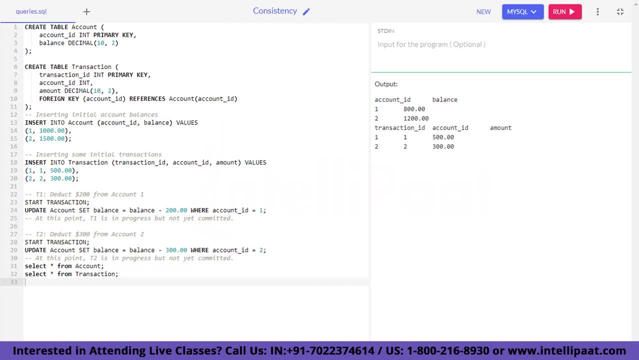 and initial balance- 1000 and 1500 respectively- in an account table. We also insert two initial transactions into the transaction table. Let's consider a scenario where two transactions, T1 and T2, are executing concurrently. T1 is a transaction where 200 has been deducted from account 1.. 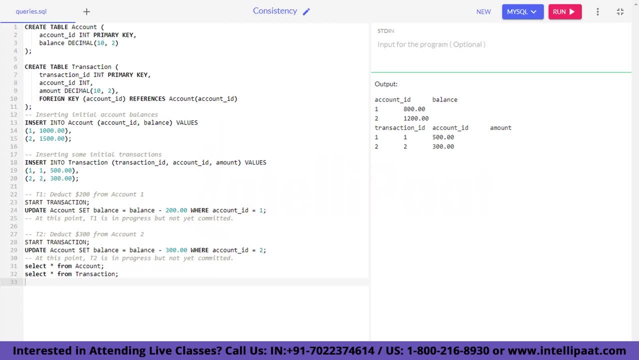 It begins the start transaction. After starting the transaction, it attempts to update the balance of the account 1 by subtracting 200 from it, but it does not commit the transaction yet. T2 is another transaction where 300 has been deducted from account 2.. 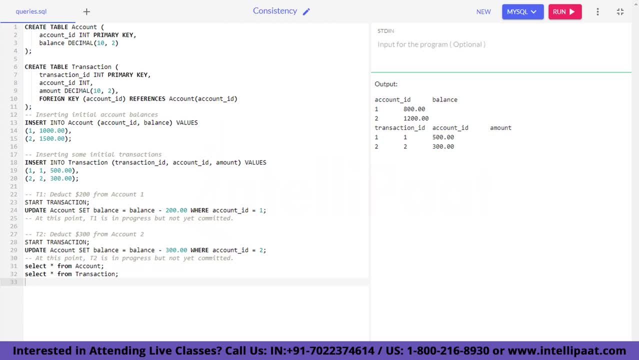 It also starts with a transaction statement. After starting the transaction, it attempts to update the balance of account 2 by subtracting 300 from it, but it does not commit the transaction yet. At this point, both the T1 and T2 are in progress but have not committed. 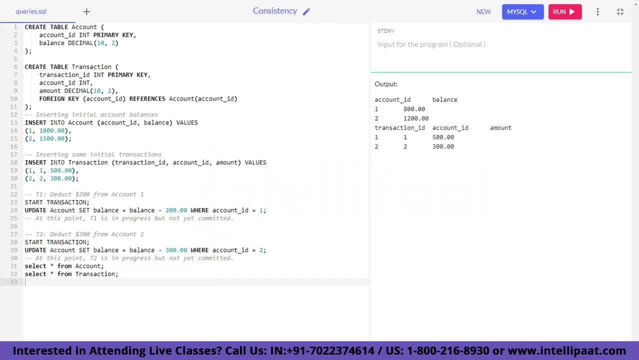 The key concept here is that they execute concurrently, meaning they are running simultaneously and can potentially interfere with each other. This is where isolation level comes into play, controlling how transactions interact with each other and ensuring data consistency. So the last property is Durability. 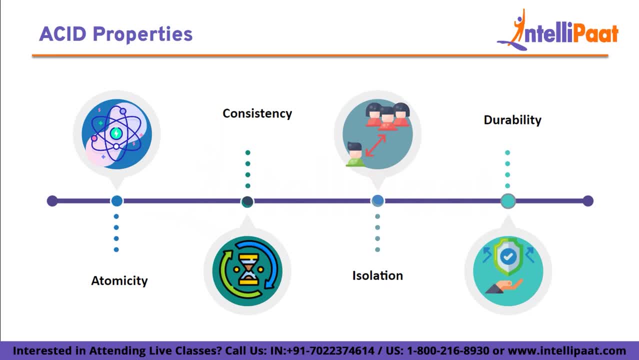 Durability comes into play when a transaction is successfully completed. Durability guarantees that once a transaction is successfully completed, changes to the database will persist even in the face of system failure or crashes. Durability means that once a transaction is closed or committed, 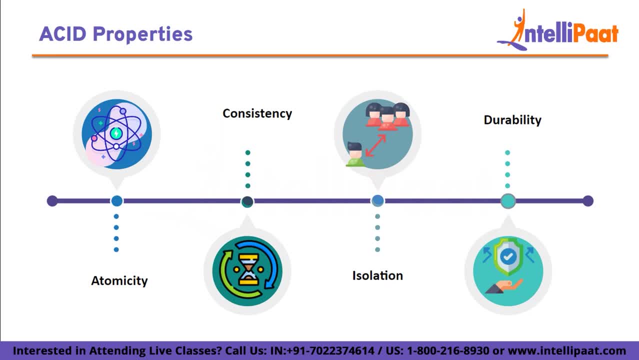 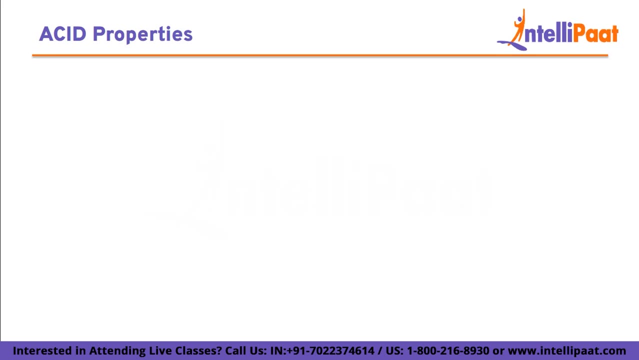 the changes made to the database are permanent. They are saved in the way that survives power outages, hardware failure or any other system crashes. When you return to the database after such an event, you will find the data just as it was when the transaction was successfully completed. 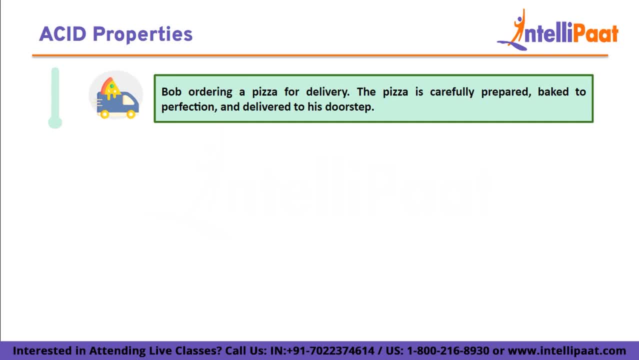 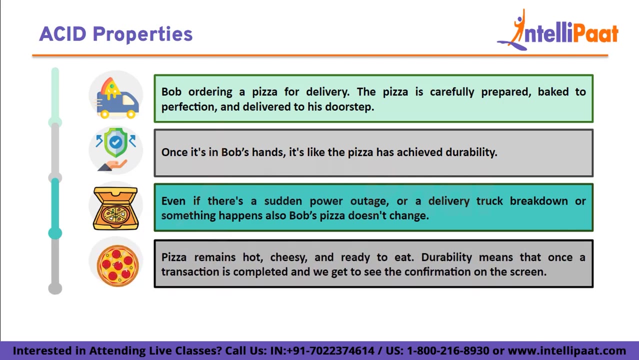 Consider Bob ordering the pizza for delivery. The pizza is carefully packed, baked to perfection and delivered to the doorstep. Once it is handed over to Bob, it's like the pizza has achieved durability, Even if there is a power outrage or delivery truck breakdown or something happens. 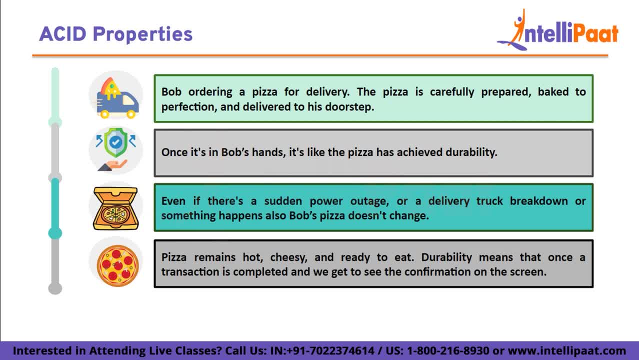 Bob's pizza does not change. It remains hot, cheesy and ready to eat. Durability means that once a transaction is completed, we get to see the confirmation on the screen that changes are made to the database and there they stay. They are recorded and stored securely. 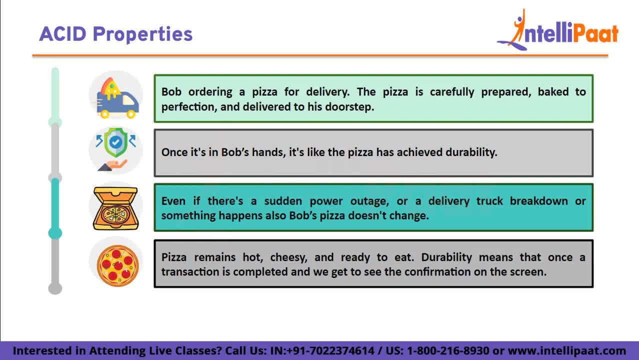 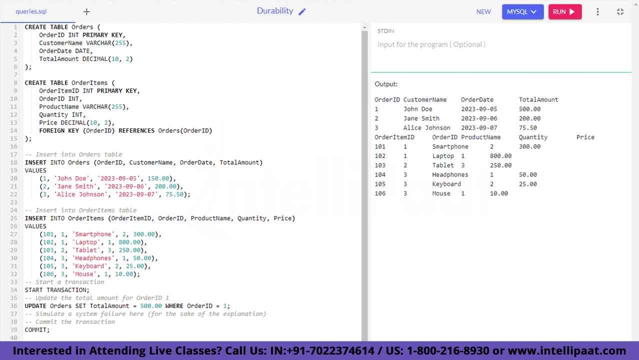 so even if there is a system crash, a server failure or any unexpected event, still data remains intact. Durability in a database transaction ensures permanent changes. We'll first create a simple database schema with two related tables: order and order item. We'll then insert some data into the table. 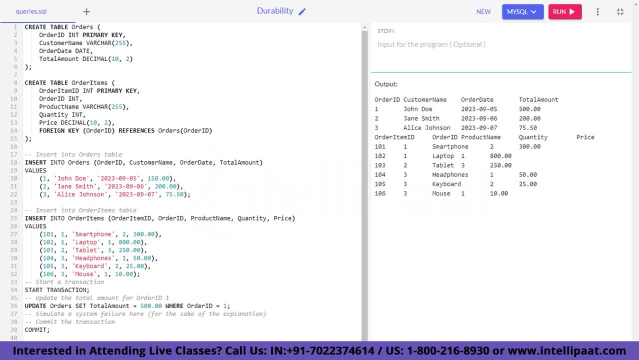 and demonstrate how durability ensures that commit changes persist even after a system failure. Suppose we want to update a total amount of order in order ID 1 to 500.. This update operation is a part of a transaction, Even if a system failure occurs after an update statement. 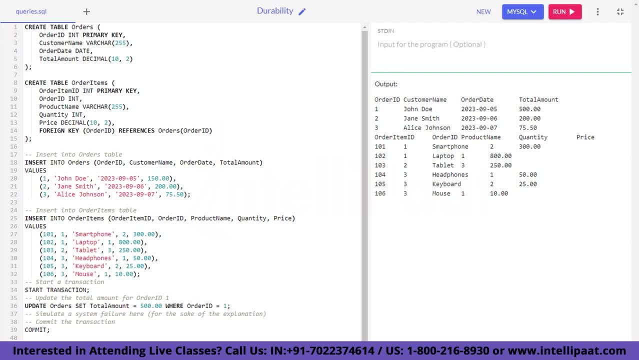 but before the commit, the database durability guarantees to ensure that the changes will still persist when the system is recovered. This is because the transaction was not yet committed, but the database logs the changes made in the way that ensures they will be applied when the system is back online. 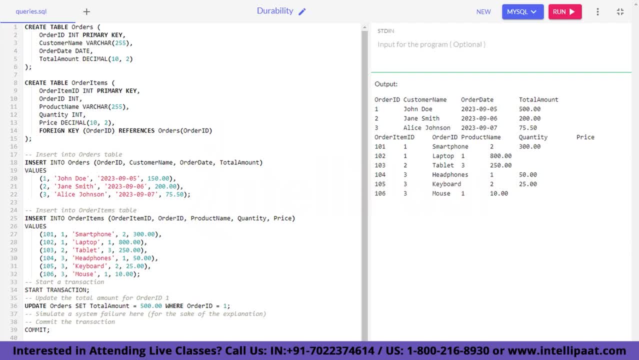 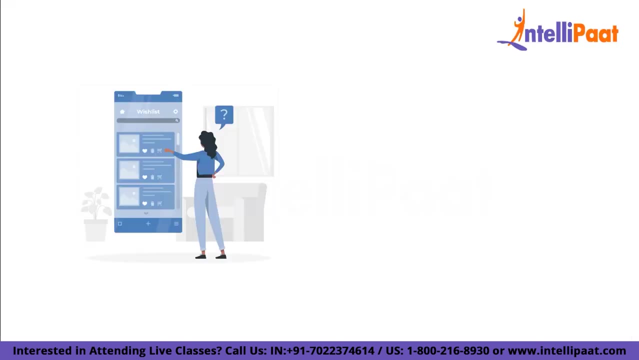 This query retrieves all the orders along with their associated item. Durability in database transaction ensures that the changes made within a transaction are persisted and recoverable even in the face of system failure, providing data consistency and reliability. Moving on, the next topic is Benefits of Asset Properties. 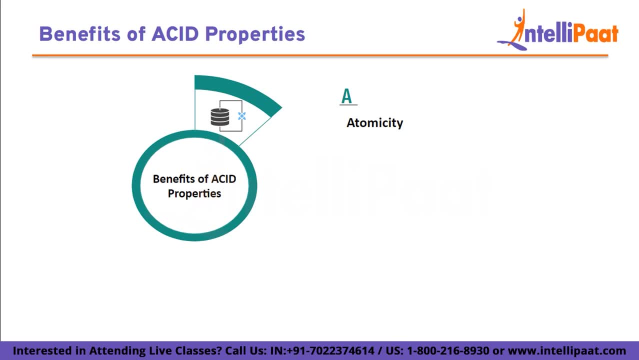 So the benefits of Atomicity is Transaction. Atomicity ensures that the series of operations within a transaction are treated as single, indivisible units. Either all the operations within a transaction are completed successfully or none of them are. This property prevents the database from being left in an inconsistent state. 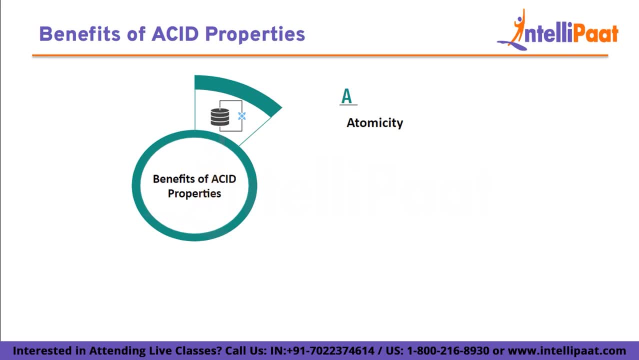 due to the partial completed transaction. Benefits include data integrity and protection against the error and failure. Benefits of Consistency is: Consistency ensures that a transaction brings a database from one consistent state to another consistent state. In other words, a transaction must follow a set of rules. 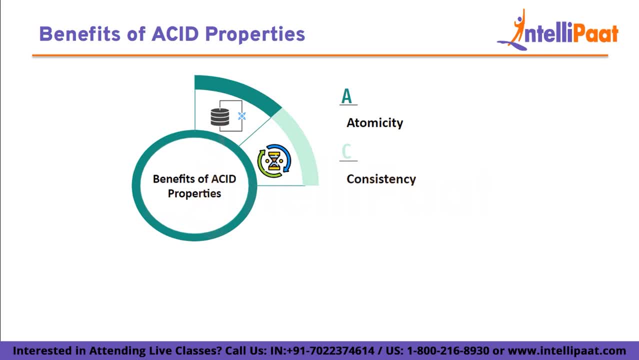 or constraints to maintain data integrity. This property guarantees that the database remains in a valid state at all the time. Benefits include data accuracy and adherence to the business rules and constraints. Benefits include improving concurrency, preventing data inconsistency due to concurrent transaction and maintaining transaction integrity. 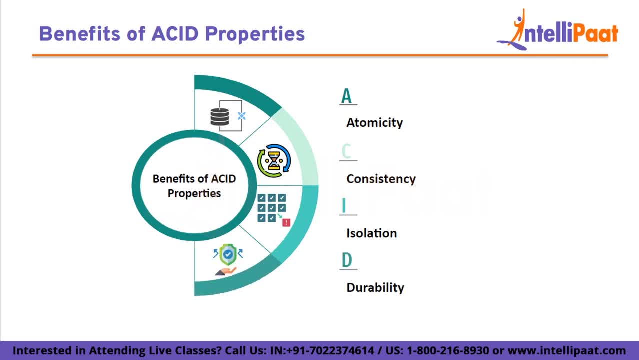 So the benefits of Durability are: Durability ensures that once a transaction is committed, it effects are permanent and will survive system failure such as power outrage or crashes. This property guarantees that data changes made by committed transaction are stored in the way that they can be recovered. 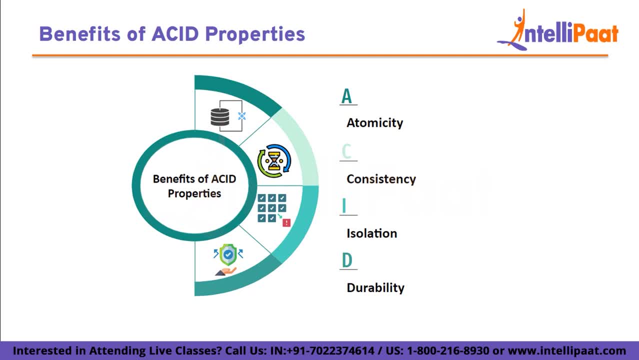 even after the system failure. Benefits include data reliability, fault tolerance and data recovery. The asset properties are fundamental for maintaining the integrity and reliability of data in a database system, making them essential for a wide range of applications, including financial system, e-commerce platform and more. 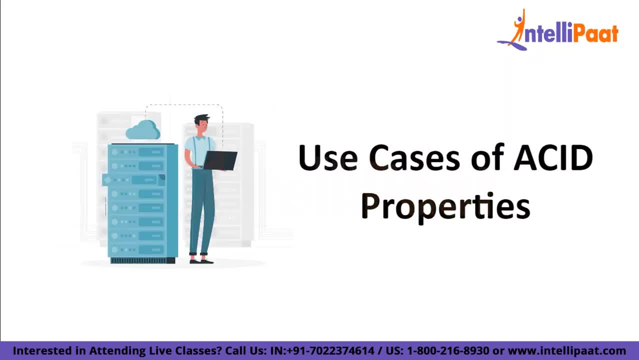 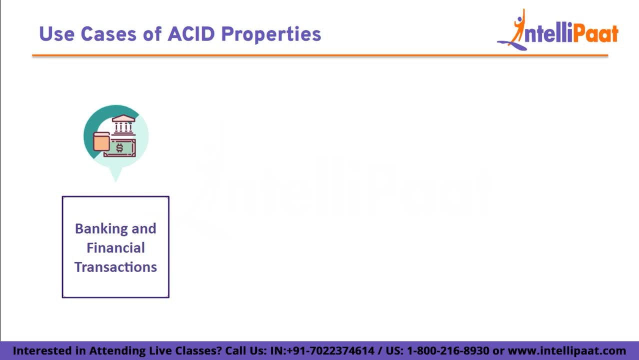 So the next topic is Use Cases of Asset Properties. The first one we have is Banking and Financial Transaction. Asset properties are crucial in financial industry. When you transfer money between the bank accounts, it is essential that the transaction is atomic, consistent, isolated and durable. 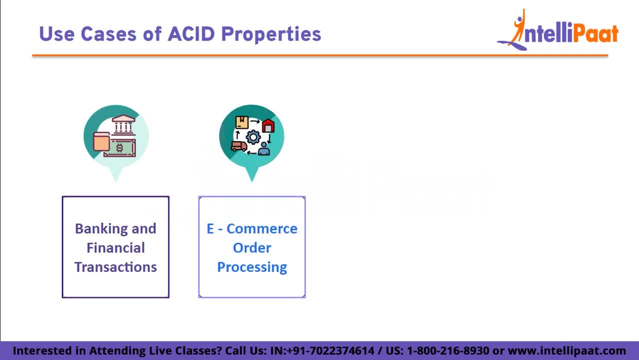 The next one is e-commerce order processing. Online retailers rely on asset properties to manage customer orders. When you place an order, the system ensures that your payment is processed correctly, inventories is updated accurately, your order does not conflict with others and the transaction is recorded securely. 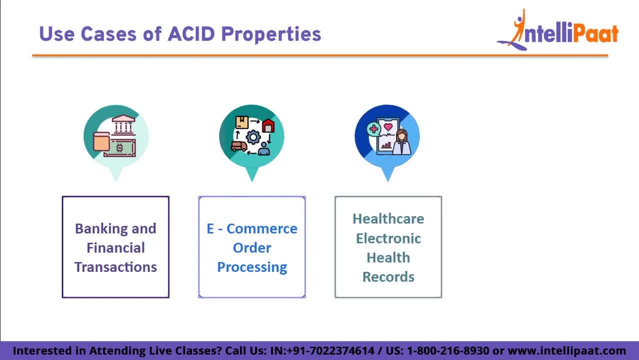 Then we have the Healthcare: Electronic Health Records. Electronic health record systems use asset properties to maintain the patient data accuracy and privacy. When a data updates your medical report, it is crucial that the changes are atomic, consistent, isolated and durable. The last one we have is: